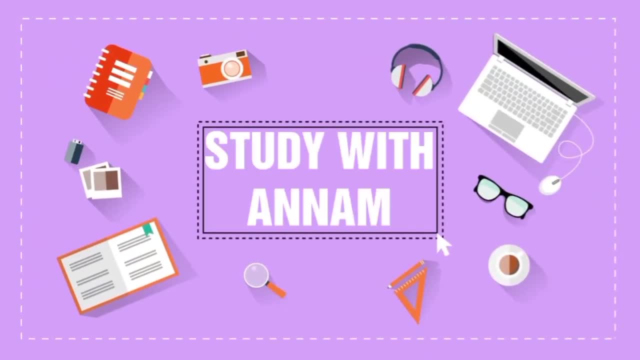 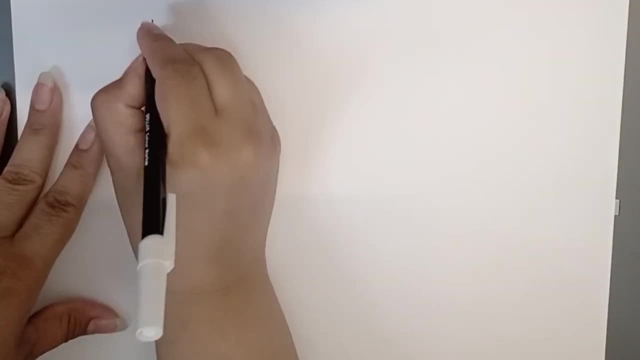 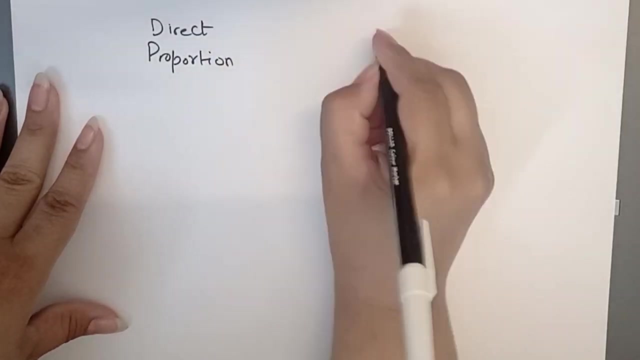 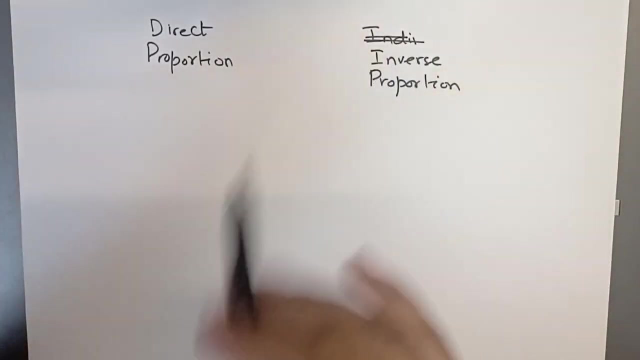 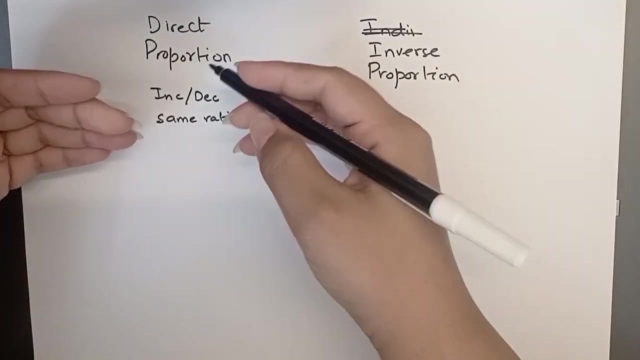 There are two topics related to proportion. One is known as a direct proportion and the next one is inverse proportion. Now, these two are completely opposite of each other: Direct proportion and inverse proportion. Now, what is direct proportion? Direct proportion is referred to a term which is increasing or decreasing in the same ratio. Basically, 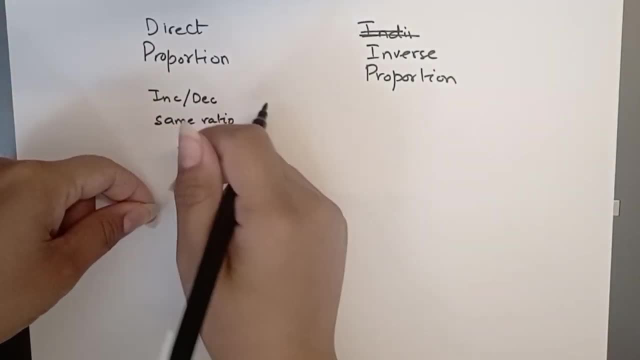 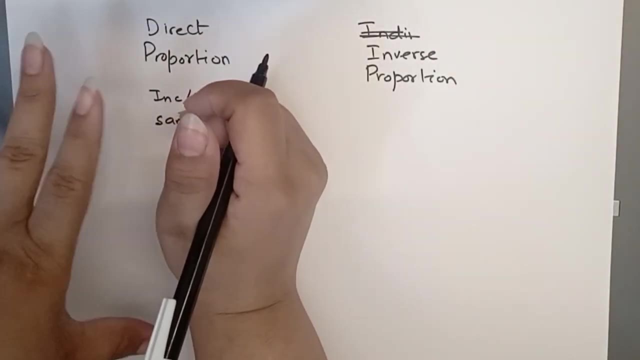 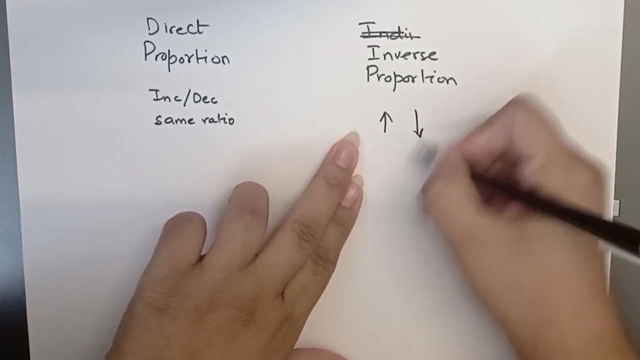 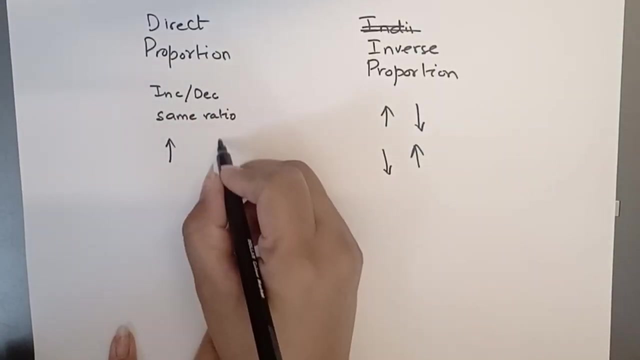 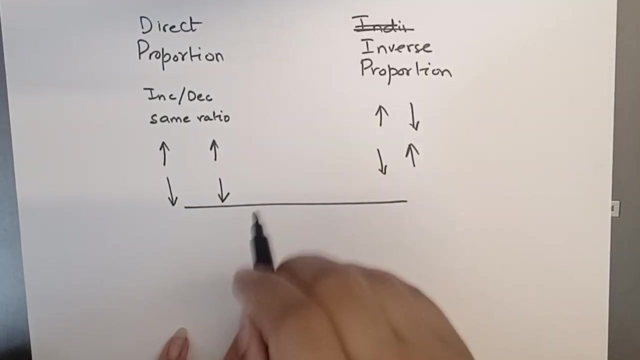 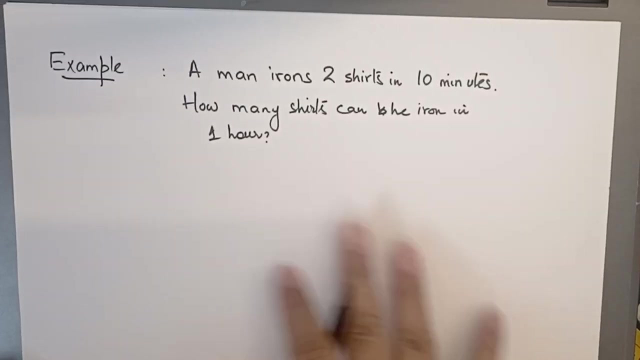 it is like if one term is increasing, then the other term will also be increasing or decreasing, then the pattern of the other will also be decreasing. I will explain it to you with the help of examples. Now here is an example: A man ironed two shirts in ten minutes. How many shirts can 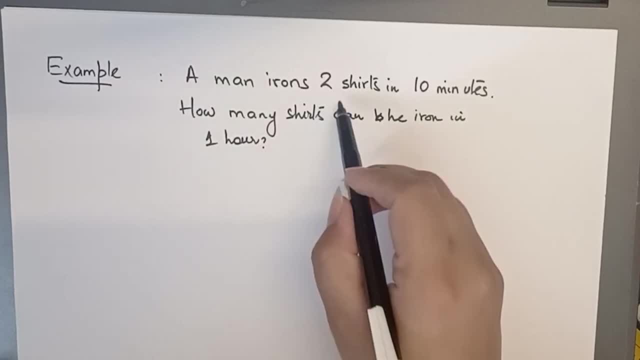 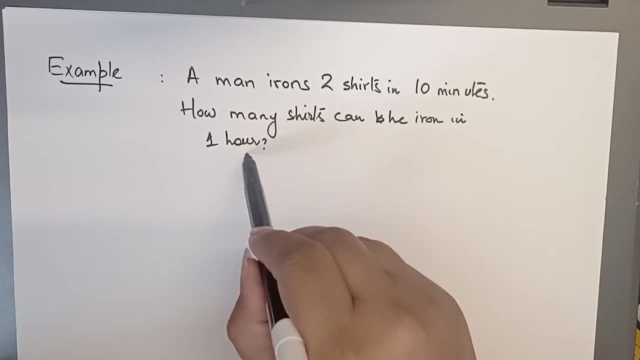 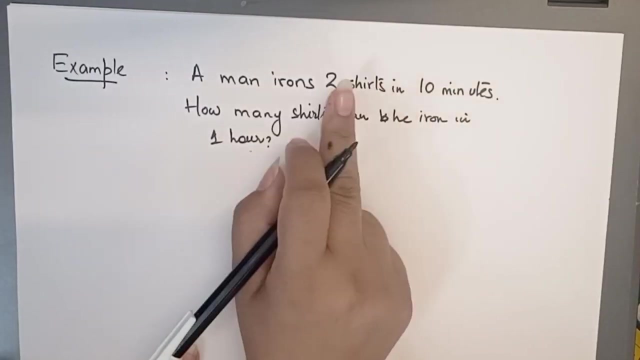 he iron in one hour. Now here is an example: A man ironed two shirts in ten minutes. How many shirts can he iron in one hour Now? this time we will write the number of shirts in two hours. Now the method is: first you will write shirts and then minutes, And the second you will 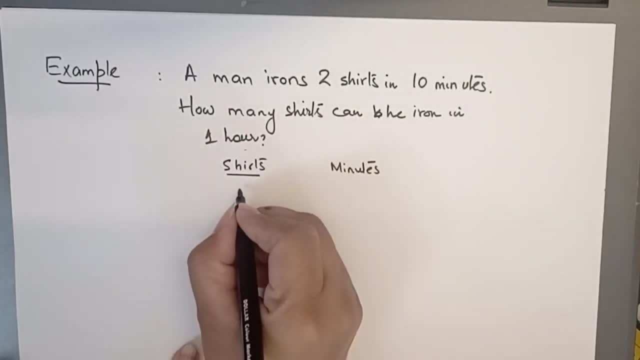 write minutes Now. how many shirts are we doing in two minutes? Ten minutes And then Now we don't know how many shirts will be there in 1 hour. If 1 hour is in minutes column, we will convert it into minutes. 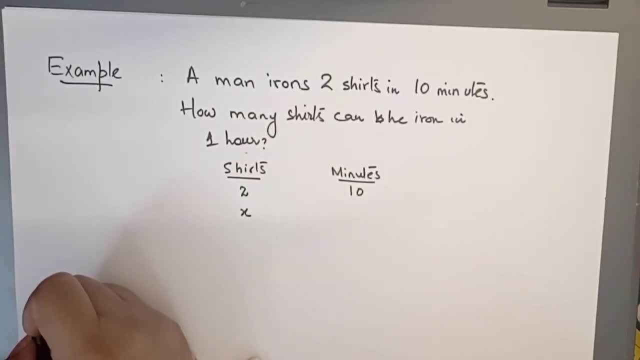 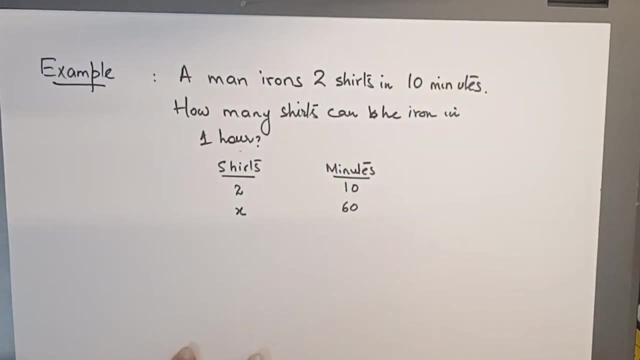 We don't know how many shirts will be there, so we will suppose it as x, And in 1 hour it will be 60 minutes. 60 minutes and 1 hour means same. If you see this ratio, then these minutes are increasing. 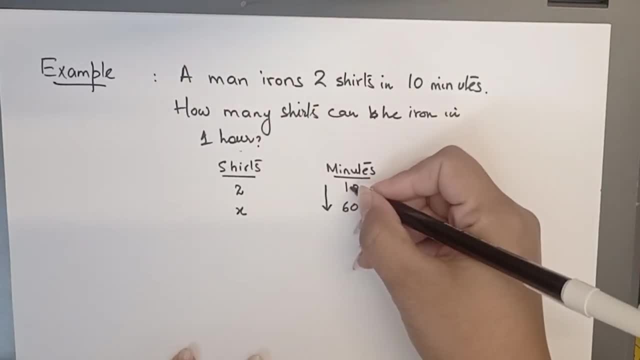 10 was before. now. for next situation it will be 60.. It means that if 2 shirts are there in 10 minutes, obviously if minutes are more, then shirts will also be more. That means this ratio will also be increasing. 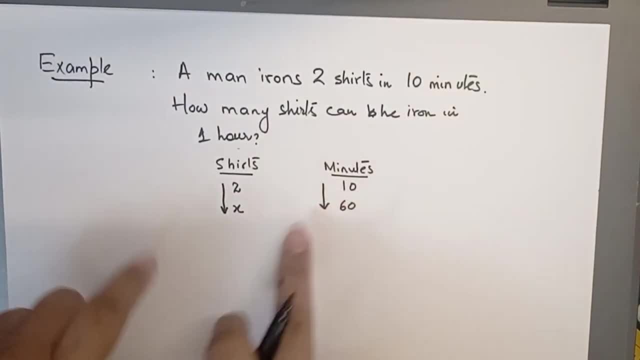 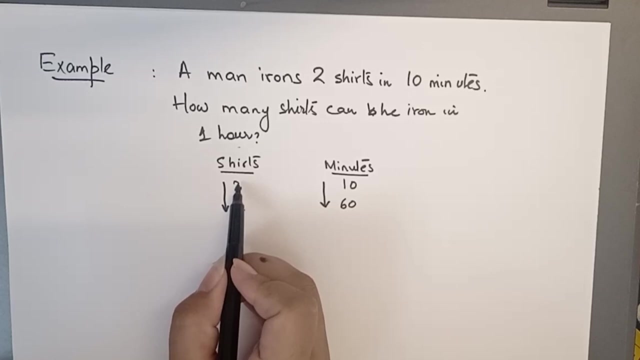 Now, how are you going to form it in the form of an equation? First, you will take it in fraction form. then you are going to do the calculation. Okay, what is its method? The tail is an arrow. From where this point is: you start writing the fraction. 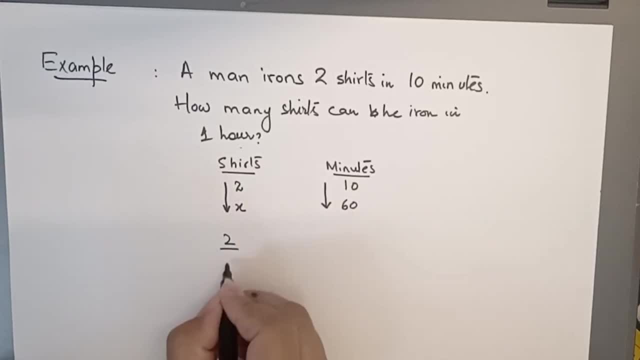 This was the first tail, so that will be like 2 upon x. Here it will be equals to. This tail was on 10,, so 10 upon 60.. Now what will happen? To solve it, you will do the cross multiplication. 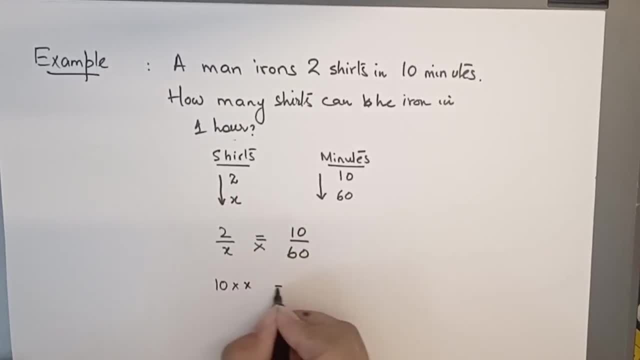 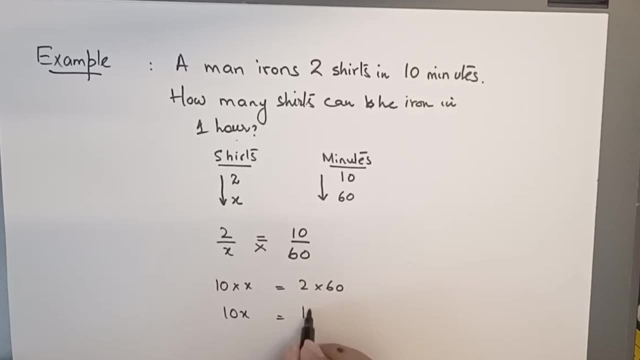 10 and x will be multiplied. 2 and 60 will be multiplied. Right, That will become: 10x is equal to 2 into 60.. 60 is 120.. Okay, Now x is here: 120 upon 10.. 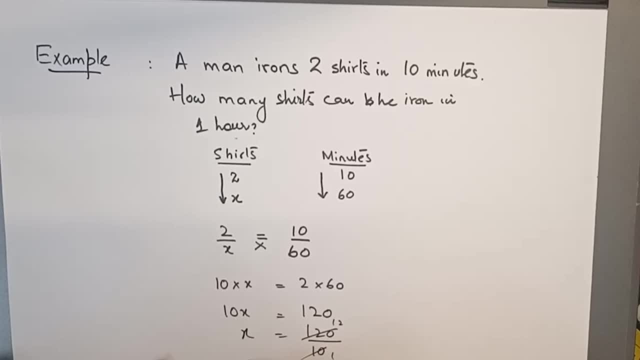 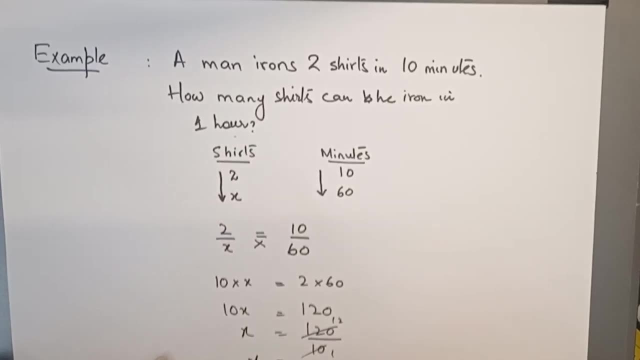 Now, both of them are 10 ones, So x will be 12.. So we got to know that write 12 shirts. So we got to know that x is equal to 12.. That means 12 shirts will be there in 60 minutes. 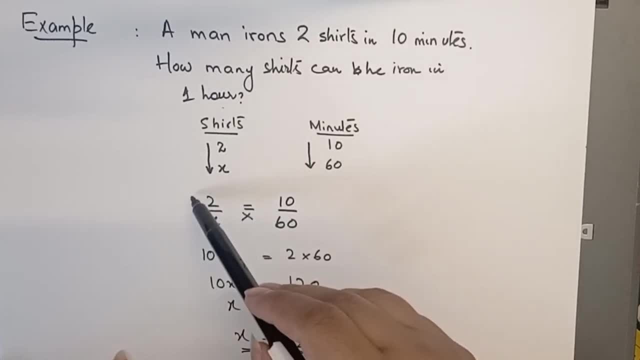 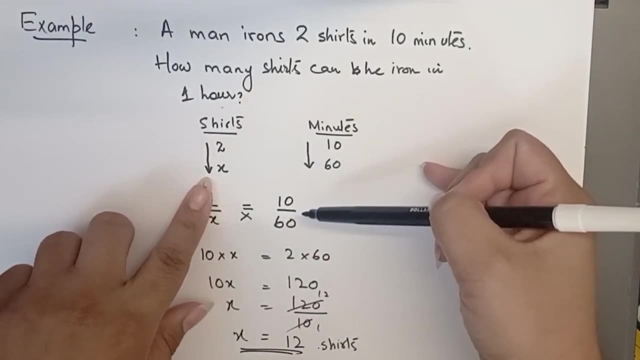 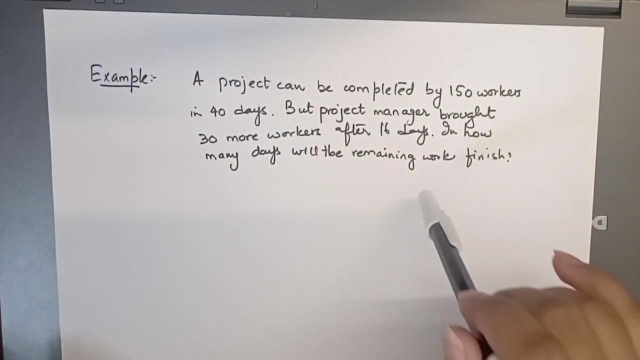 Right, So this is how you calculate. Now, this case is a case of direct proportion, Because when one term is increasing, the other is also increasing. Okay, Okay, now let's consider this example. This example is of inverse proportion. 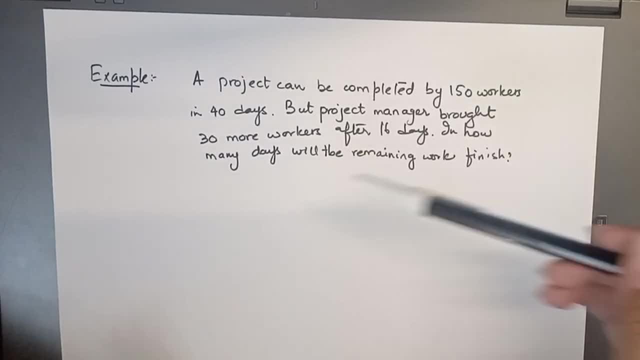 Inverse proportion means if one term increases, the second term will decrease. Okay, A project can be completed by 150 workers in 40 days. 150 workers is a project which can be completed in 40 days, But project manager brought 30 more workers after 16 days. 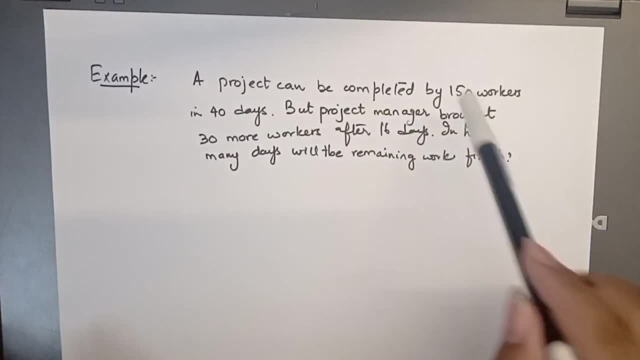 How many days will the remaining work finish? Okay, Now the thing is that after 16 days, the project manager brought 30 more workers. Okay Now. first it was 150.. In that, 30 were added, Right. 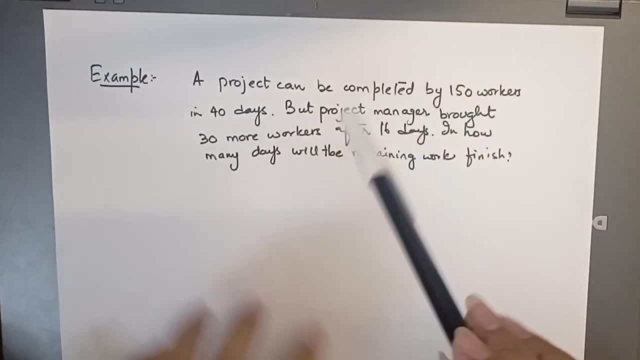 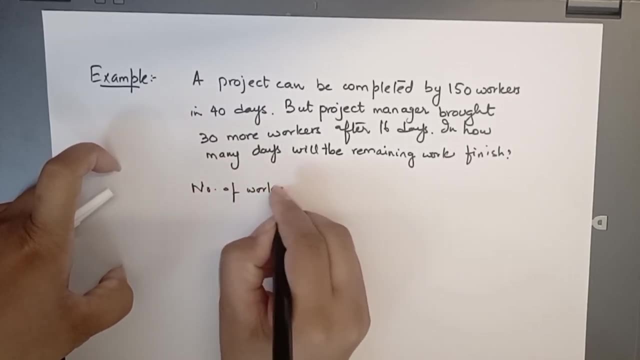 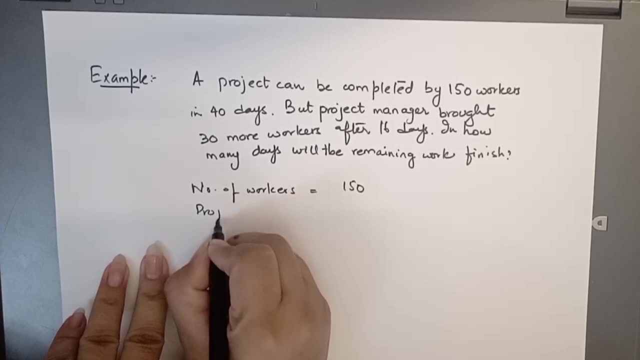 Now, in how many days will the remaining work finish Now? how many days will the remaining work finish? Now? we know that the total number of workers you had was 150. Okay, They were 150. Okay, And how long did the project completion take? 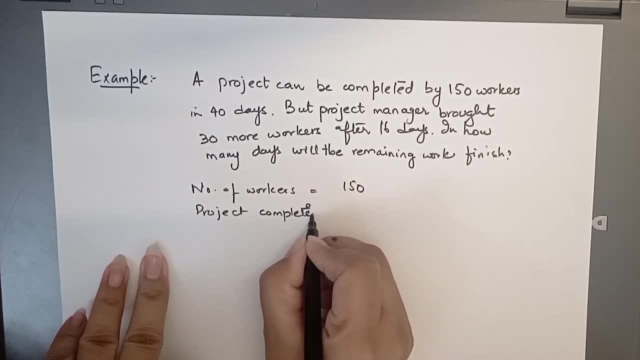 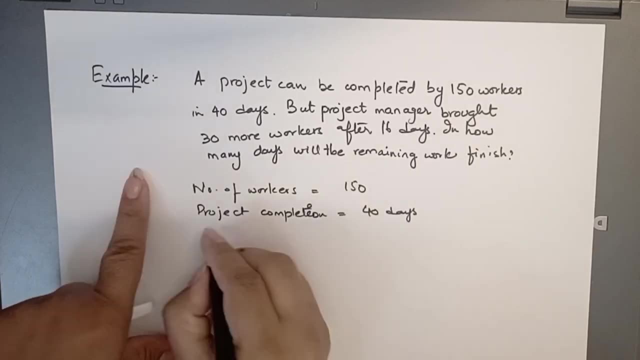 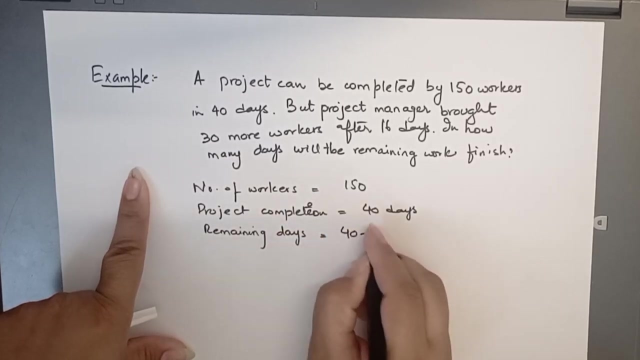 The project completion was completed in 40 days. Now, how many remaining days do we have? We have worked in 16 days. Okay, The remaining days will be 40 minus 16, which will be equal to 24 days. Okay. 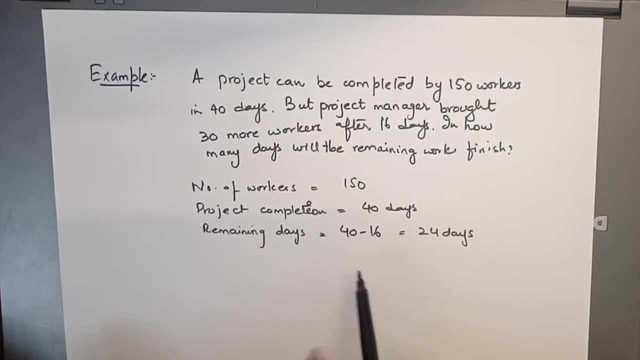 16 days. Okay, So from the 40 days they worked, how many days will be left? 24 days Now, when there were 24 days. the remaining work of 150 workers can be completed in 24 days. 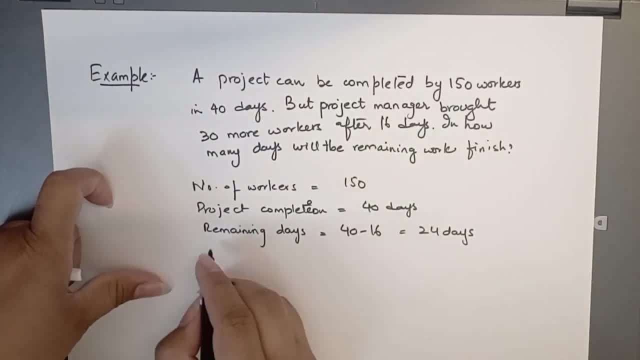 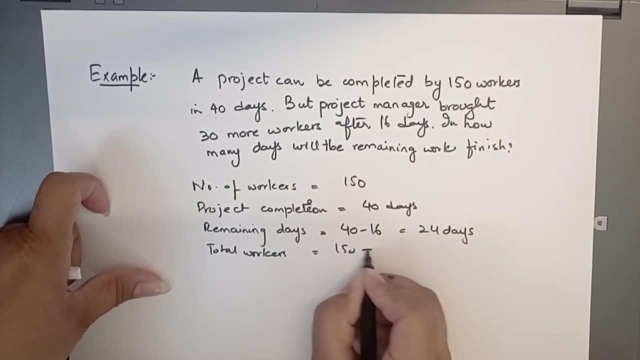 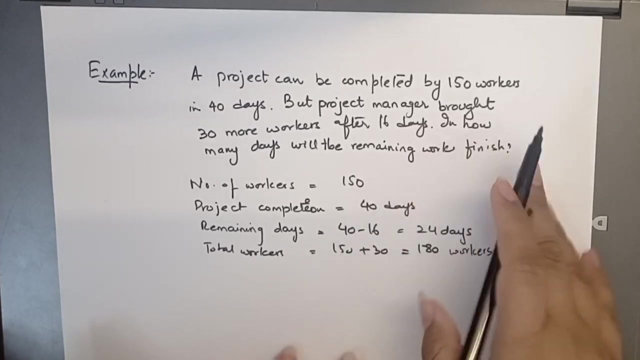 After 16 days, they brought 30 more workers. Okay, Now, how many total workers do we have? 150 plus 30 is equal to 180 workers. Okay, We have 180 workers. Now we have to see how many days will be left. 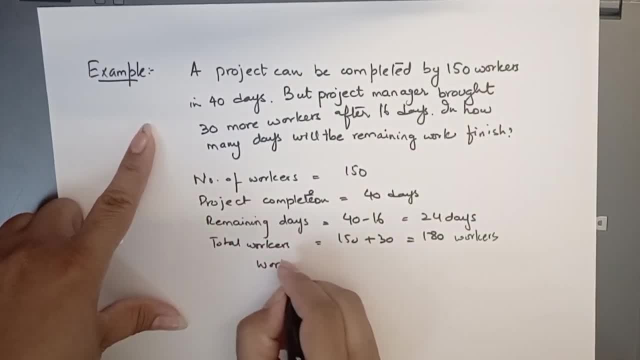 Now you can see the ratio of the days. Now you will make a column of the same ratio. One term is coming for the workers. one term is coming for the days. Now the remaining work is being completed. There are 150 workers. 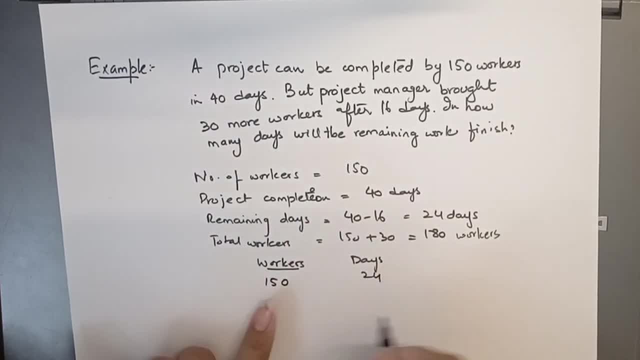 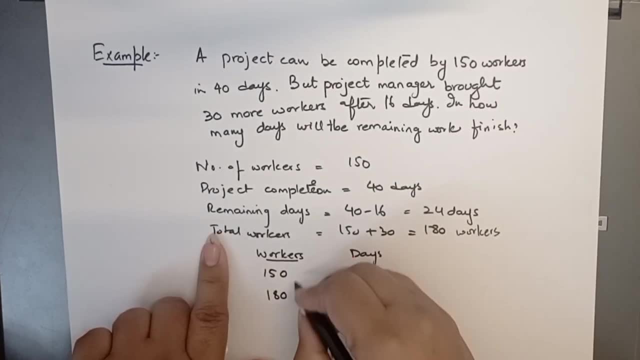 They can complete the rest of the work in 24 days. Okay, What happens if 180 workers come? how many days will they work? Now here you see that the term is increasing. There were 150 workers. they have increased to 180.. 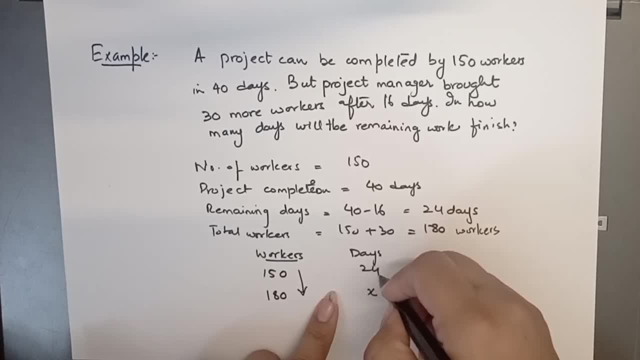 If 150 workers were working in 24 days, then there is an obvious thing: The 180 workers will work very fast. Obviously, when there is more manpower, then the work will be completed very fast. It means that your days will be less. 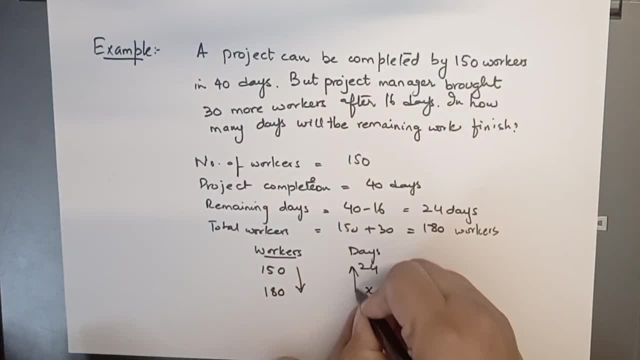 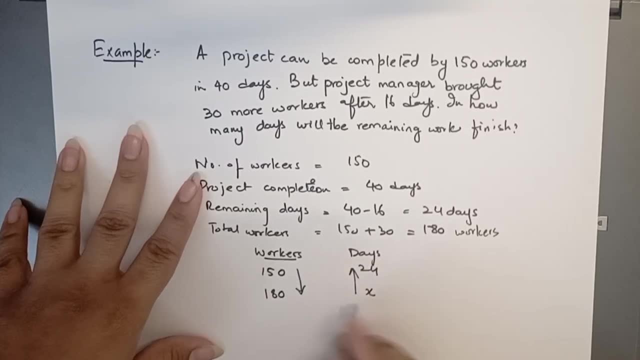 So the sign of your arrow will come from upwards. Okay, Okay Now. now, the same thing is that you have to make a fraction from the tail of the arrow. That will be: 150 upon 180 is equal to. the tail of the arrow is here: x upon 24.. 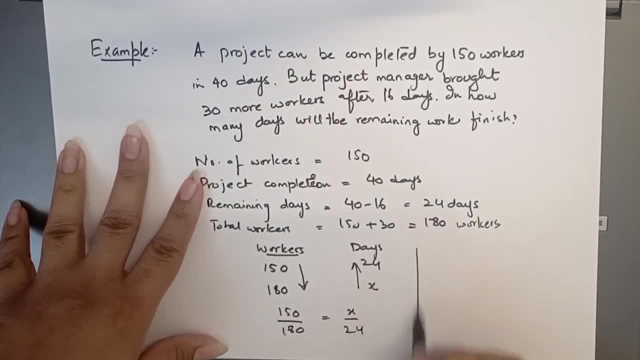 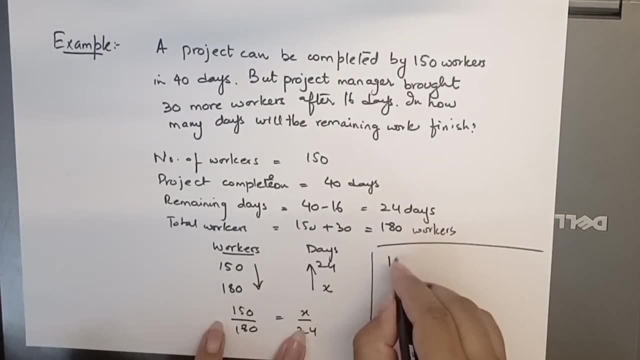 Okay, Here I am solving the rest because I don't have place. Okay, Okay, Okay, Now here you see. you do the cross multiplication: 180 x x is equal to 150 x 24.. Okay, You take x here, 150 x 24, which is so big, you multiply it and get the answer. 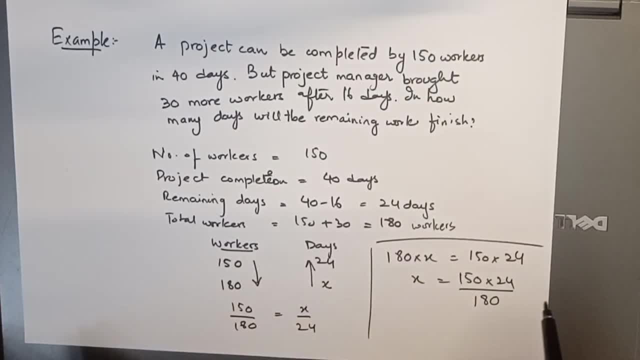 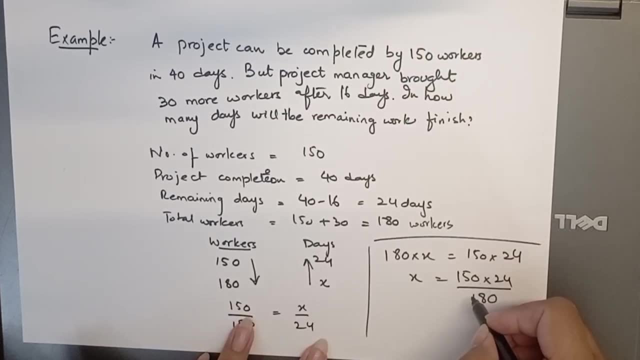 You cut it like this: Okay. Okay, Now we know that if we go from its table, it is cut from 0, 0.. Okay, Now we know that if we go from its table, it is cut from 0, 0.. 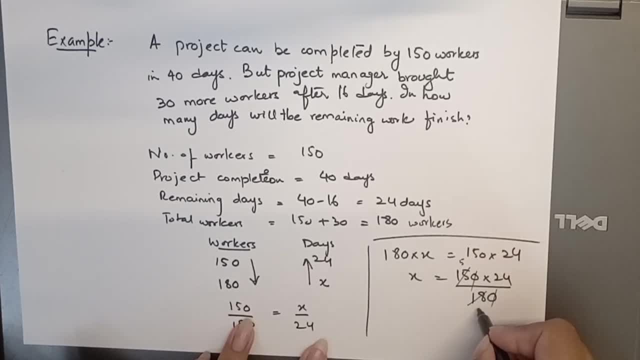 Okay, Then what do we do? We go from the table of 3.. 3- 5s are 15, 3- 6s are 18.. Okay, Now we know that 6- 1s are and 6- 4s are 24.. 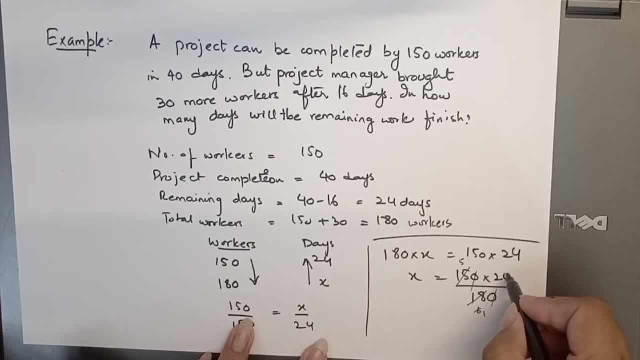 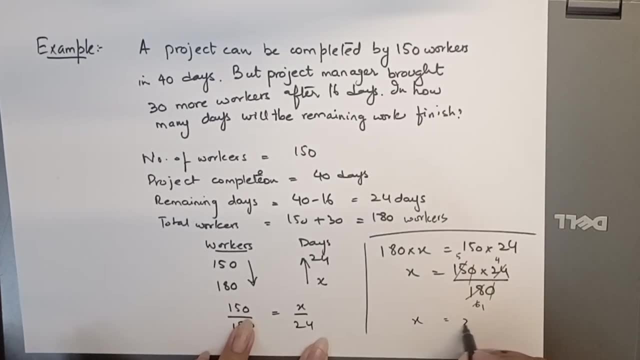 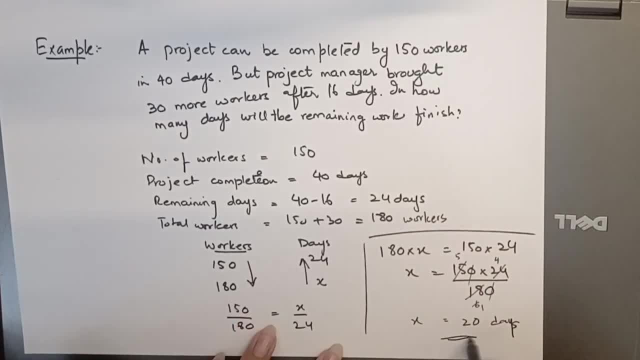 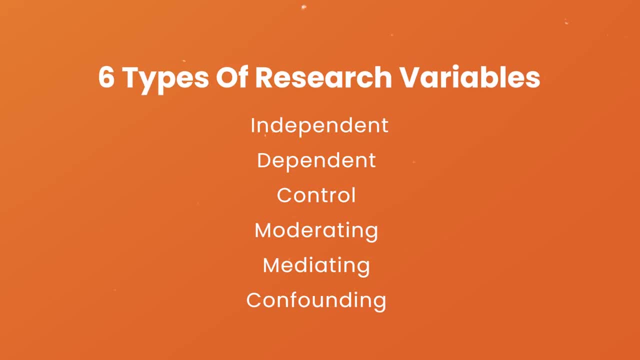 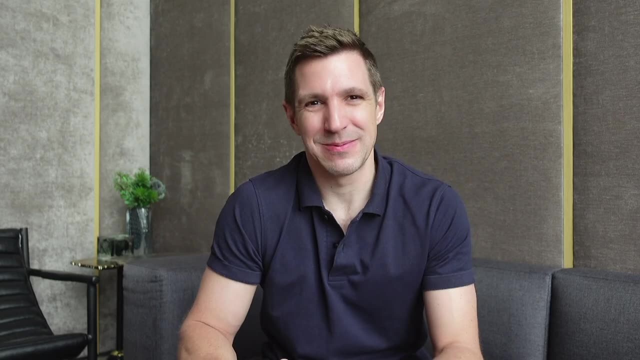 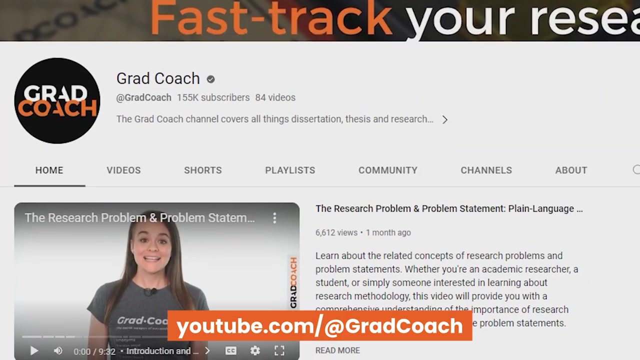 In this video we're going to unpack and explore six different types of research variables, that you can understand what they are and how to use them correctly. Let's do it. Hey, Derek here from Grad Coach. If it's your first time here, the Grad Coach channel is where. 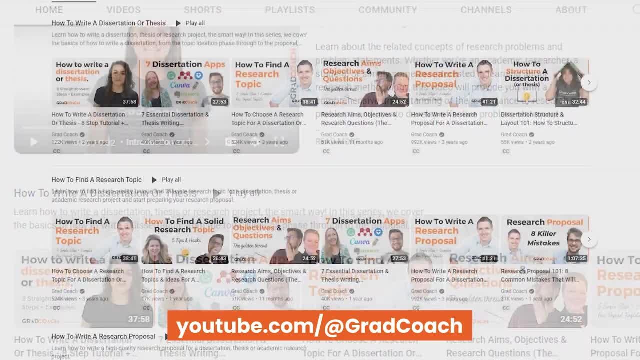 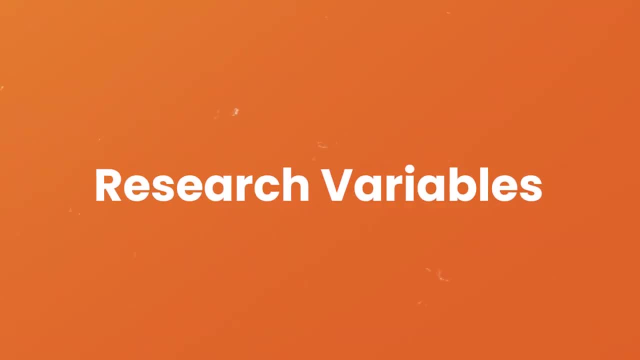 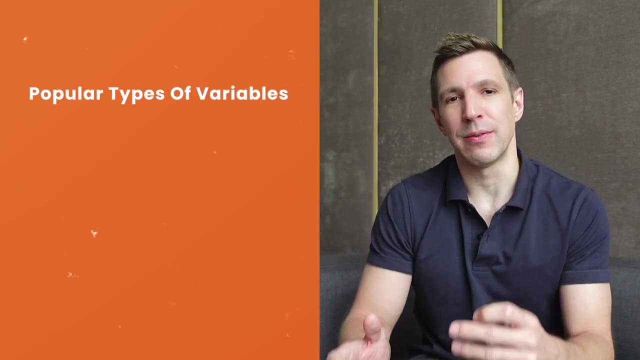 we discuss all things research related so that you can approach your project with confidence and competence. In this video we're going to dig into the topic of research variables. We'll start by first explaining what a variable is, And then we'll look at six popular types of variables. 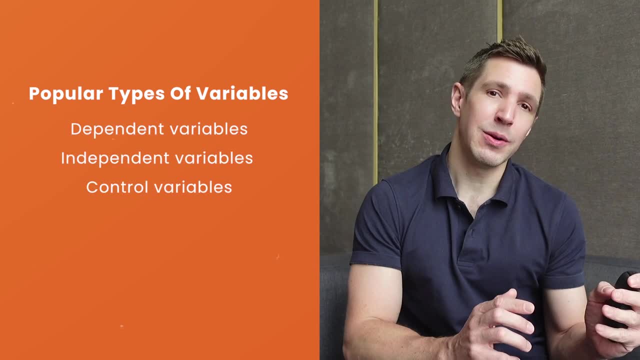 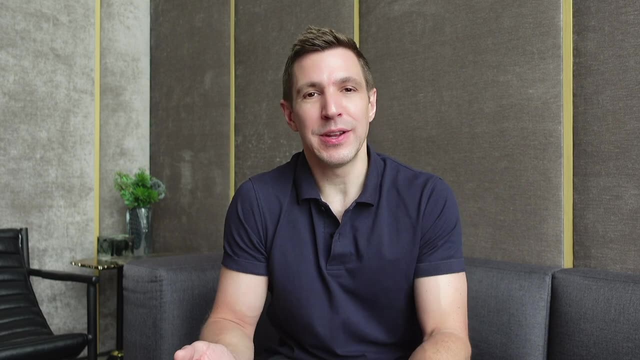 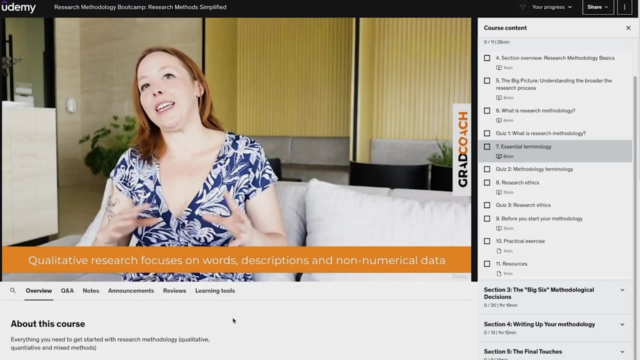 specifically dependent, independent and control variables, And then we'll look at moderating, mediating and confounding variables. It's worth quickly mentioning that this video is based on an extract from our popular online course research methodology boot camp. If you are new to formal, 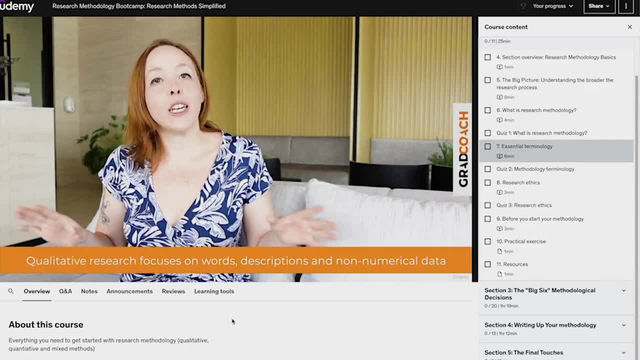 academic research. you definitely want to check that out And to say thanks for watching this video. we've got a lot more content coming your way. Don't forget to subscribe to our channel and turn on notifications, And I'll see you in the next video. Bye.